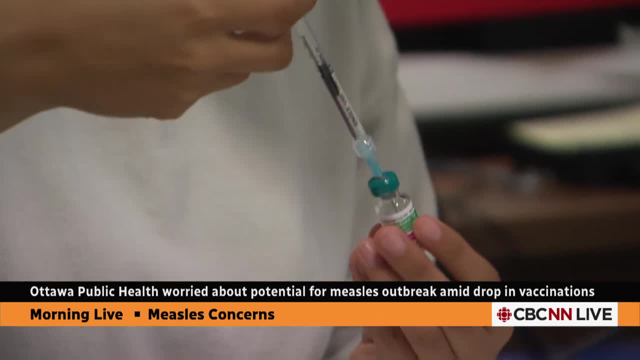 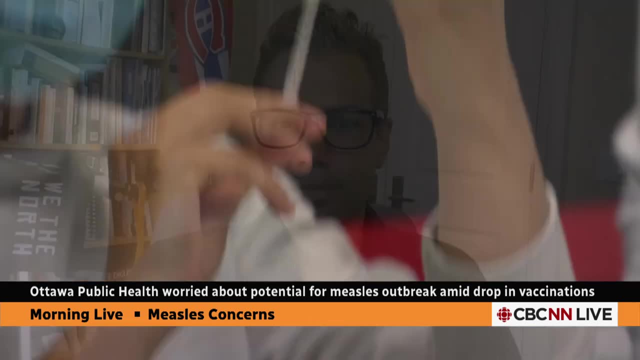 rashes fever cough, But in 10% of cases of measles there can be complications including pneumonia and encephalitis. Let's bring in Dr Samir Gupta. There's a starting point for our conversation with Dr Gupta this week. a respirologist and an associate professor. 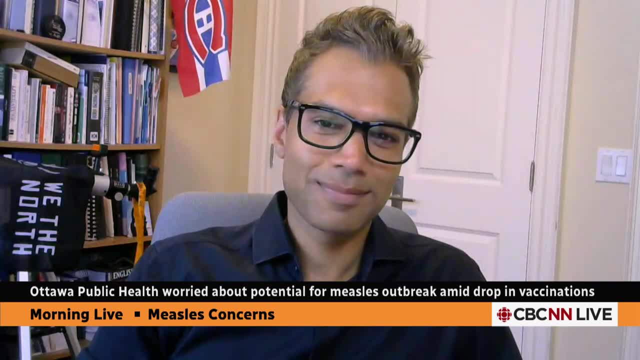 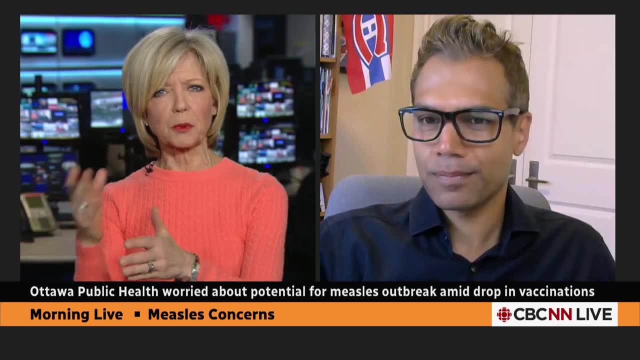 with the University of Toronto. Good morning Dr Gupta, Morning Heather. I'm wondering the timing of this. it was interesting just the start of March. but looking ahead to March break: more mixing, more travel. So Ottawa's public health warning about. 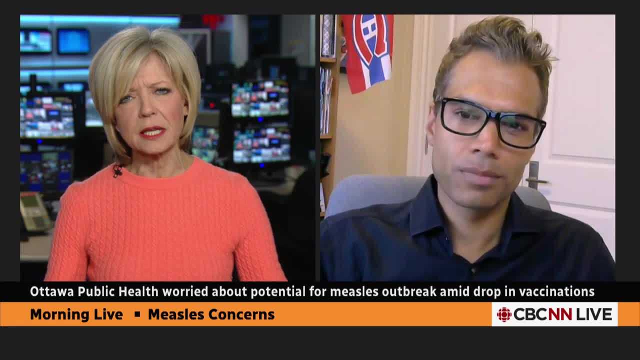 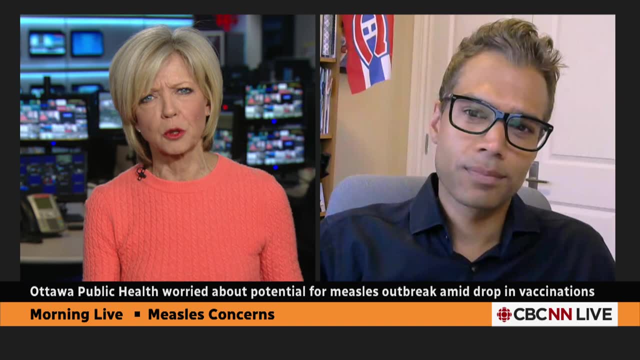 the potential for a resurgence of measles and they're putting together a team to get set for any potential outbreaks. Why are we seeing a resurgence of measles, Dr Gupta, and what should parents know? Yeah, you know. so the why is similar to 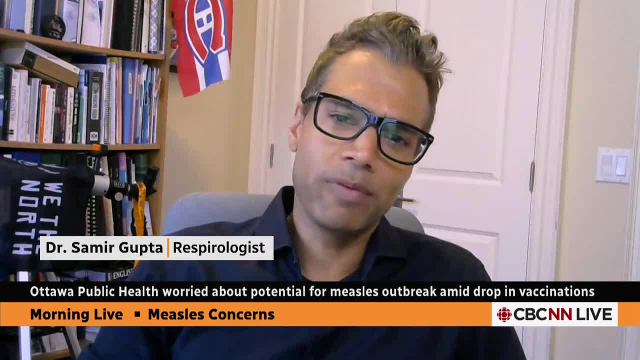 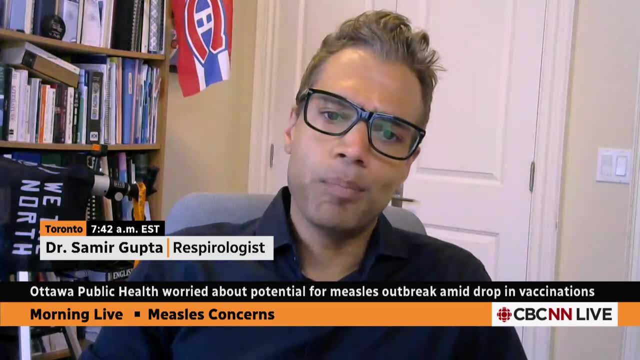 I think we talked about polio coming back and you know we've heard in the last few years of outbreaks of mumps and these are all diseases that we had largely conquered with very effective vaccines but vaccine uptake has been going down and that was happening before the pandemic. 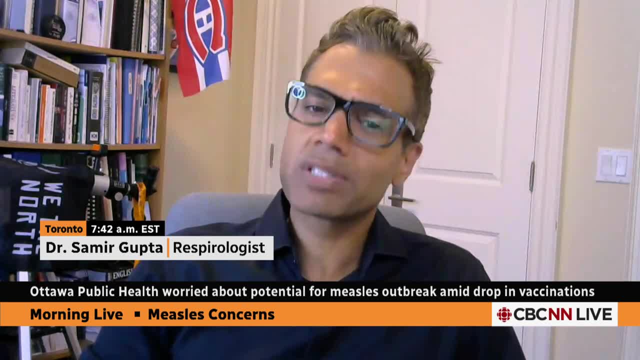 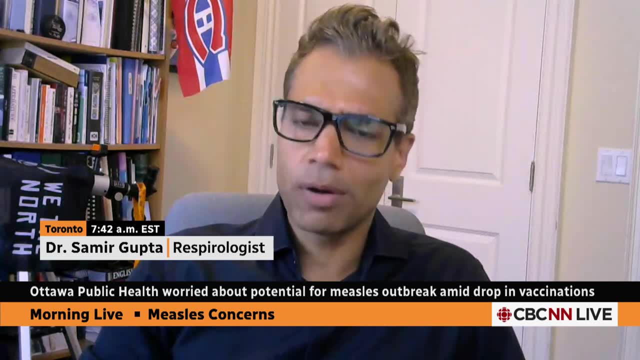 and then, as you heard in that report, a lot of people missed their vaccines, A lot of kids missed routine immunizations during the pandemic, just because of disruption with access to health care, in some cases because of increasing vaccine hesitancy. and so when you have a whole bunch of 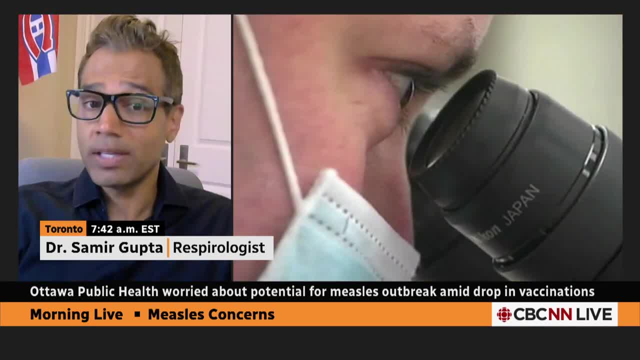 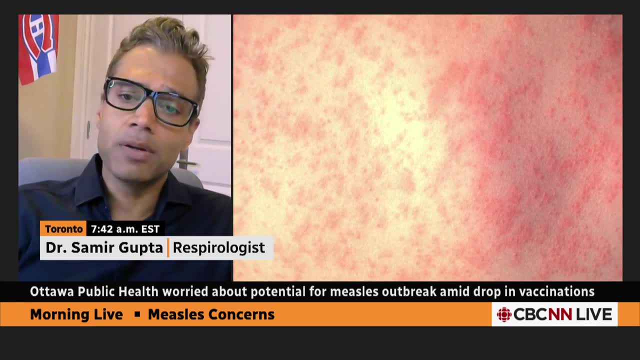 children, millions around the world who are not vaccinated against a disease like measles. you will see this disease coming out and there are outbreaks around the world and you know. so that's that's probably the why and we- hopefully we can catch up on that and get folks immunized again. 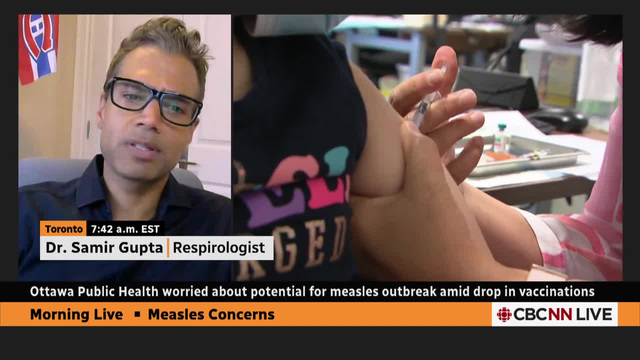 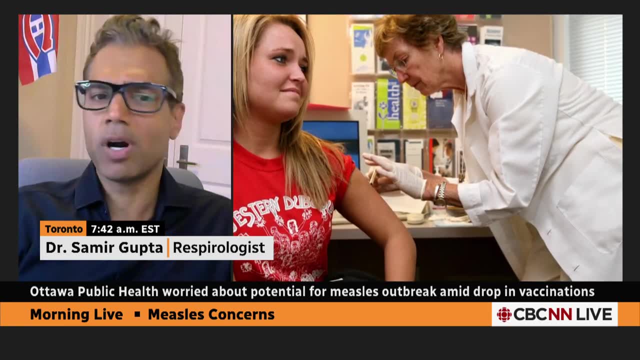 And then in terms of what parents should be concerned about, it's what you said, and the tricky thing with measles is that it behaves like any viral illness, at first with sort of cough runny nose. you do get runny eyes as well. 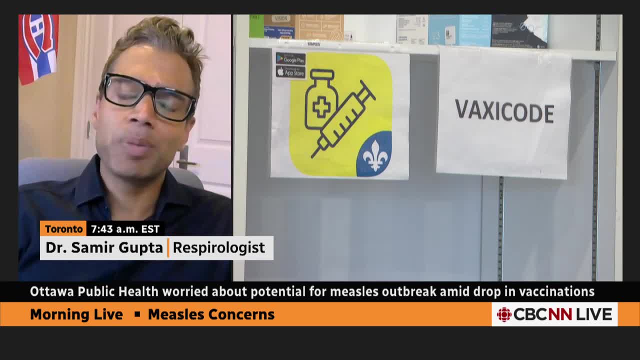 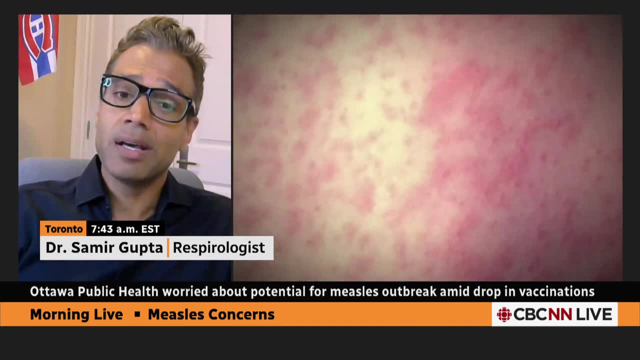 runny nose. you do get runny eyes as well, But then you have this rash which is as you showed it there. it's a telltale rash, and that's when you start thinking: oh, this is something different. but unfortunately, you are often infectious, contagious, for several days before the rash appears and then, of course, for several days.